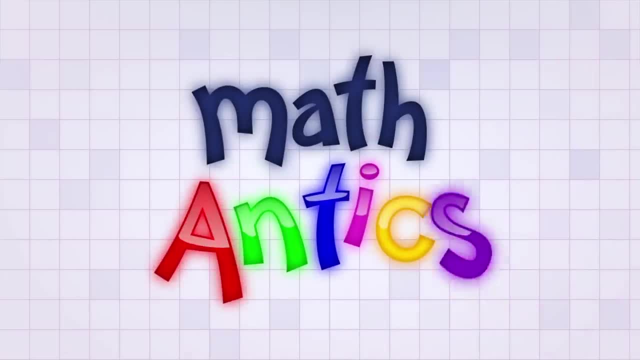 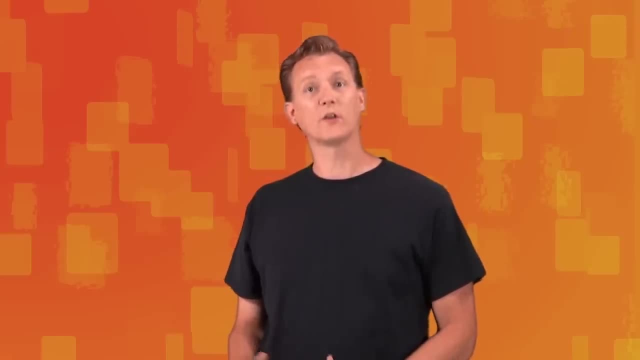 Hi and welcome to Math Antics. In this video lesson we're going to learn how to do basic multi-digit multiplication. Now this can be tricky at first, but don't get discouraged. It just might take some extra time and practice, but you'll get the hang of it. 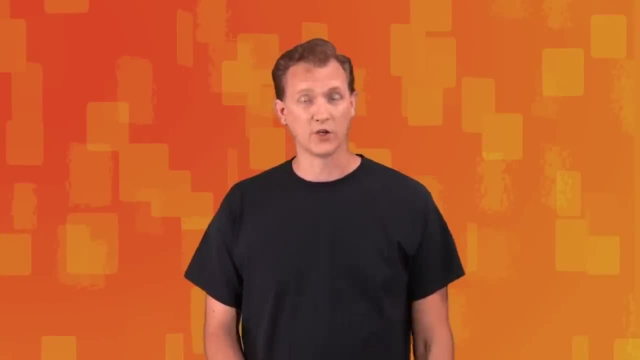 One thing I want to mention before we start is that multi-digit multiplication will be much easier for you if you memorize your basic multiplication facts. But if you don't have them memorized, then be sure to have a multiplication table handy when you're. 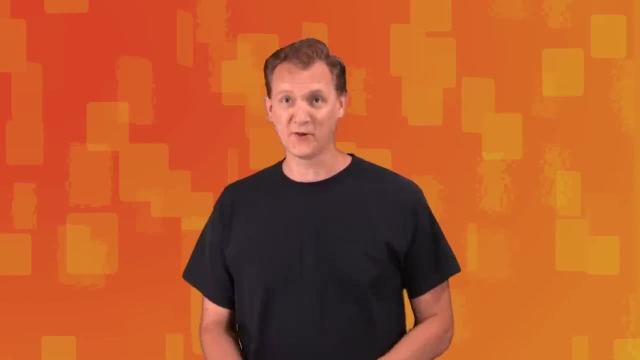 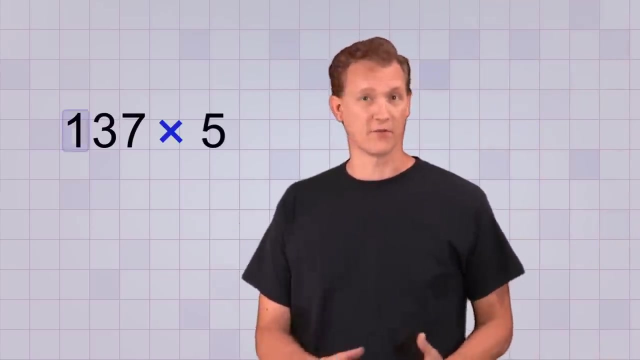 doing your practice problems. Okay, the best way to learn this is to jump right in. Let's try 137 times 5. Now, as you can see, this is a 3-digit number times a 1-digit number When you're given a problem. 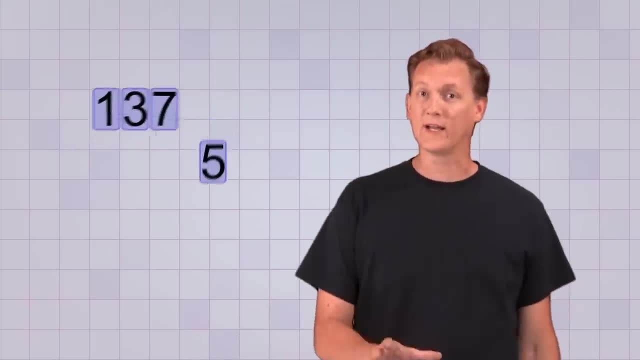 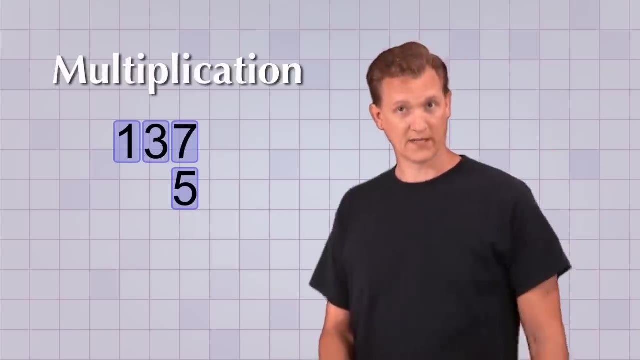 like this, where the numbers are written side-by-side. you need to rewrite it in stacked form, With the ones places lined up just the way we did with addition and subtraction. Now you might remember with multiplication that the order of the problem doesn't matter, so we can put whichever number we want on. 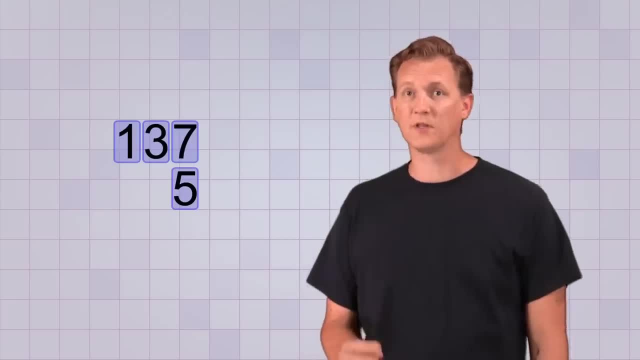 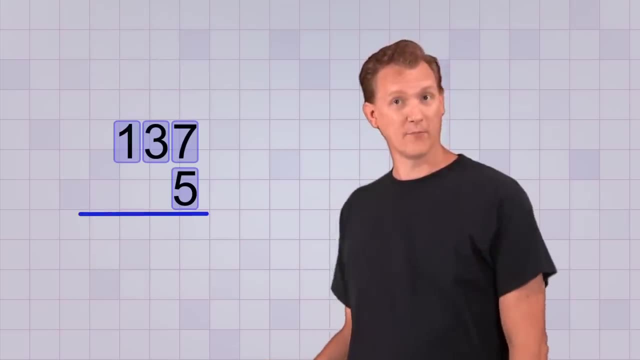 the top or the bottom, But it's always best to put the number with the most digits on the top and the one with the fewest digits on the bottom. There now we draw our answer line below and we put our time symbol to the left. so 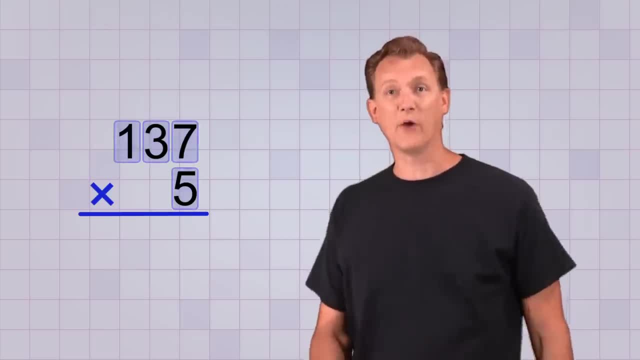 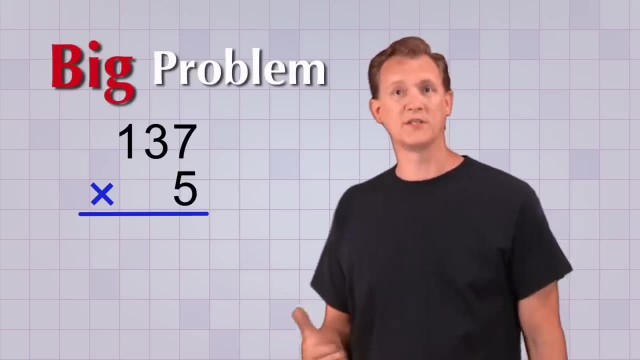 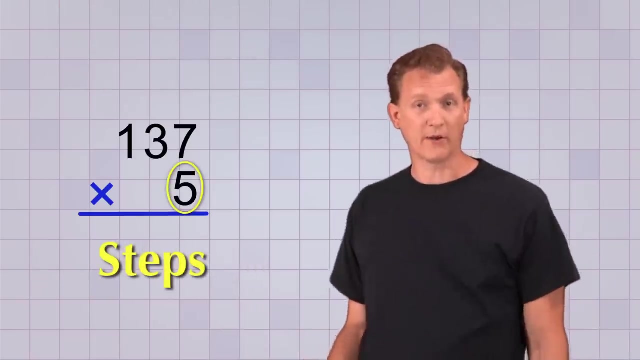 we don't forget that we're multiplying. Okay, now we're ready to learn the procedure for multiplying Basically. what we're going to do is break up this big multiplication problem into a series of small multiplication problems or steps. Those small steps involve multiplying a digit in the bottom number by 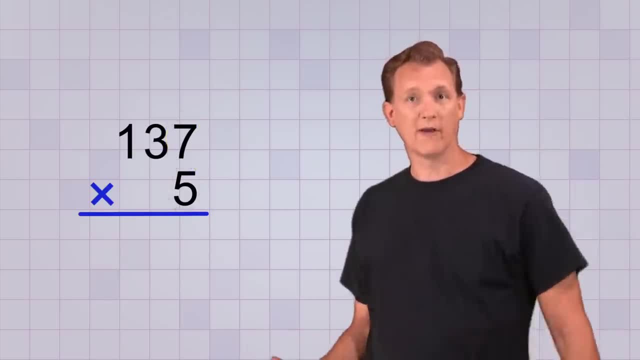 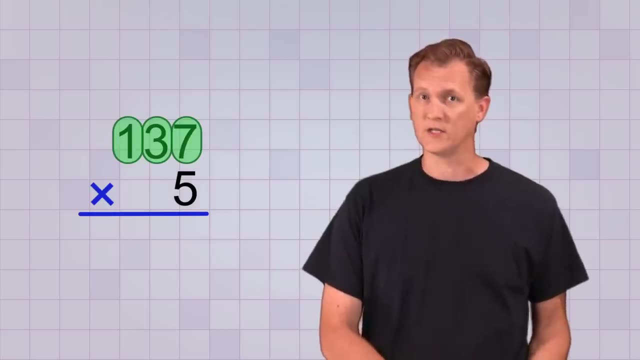 a digit in the top number. Now in our problem we only have 1 digit on the bottom and we're going to multiply it by each of the digits in the top number And since the top number has 3 digits, that means that our problem will have 3 small multiplication steps. 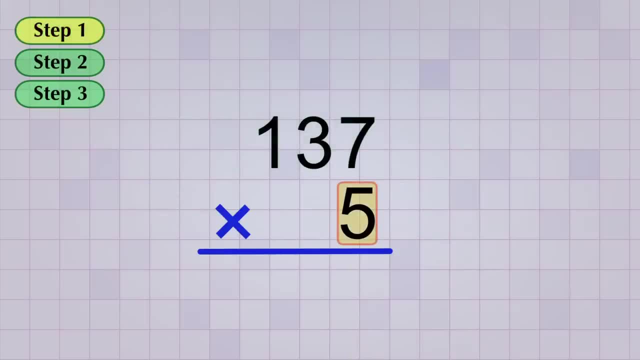 For the first step, we multiply the bottom digit, 5, by the digit in the 1-digit number. Now in the ones place of the top number, which is 7, we always start with the ones place and work our way from right to left. So 5 times 7 gives us 35.. 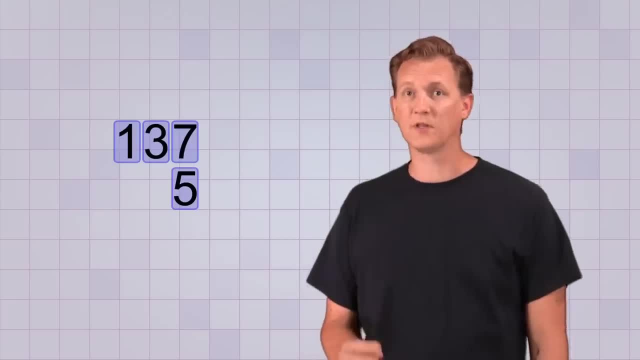 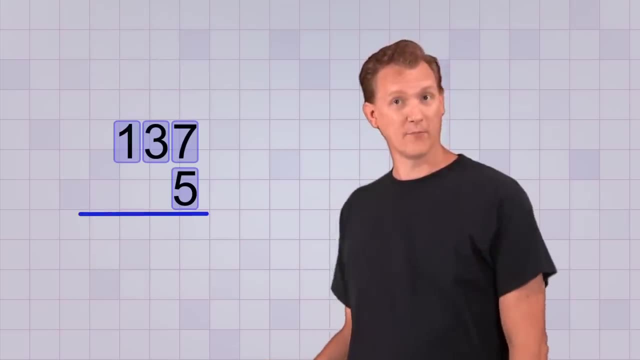 the top or the bottom, But it's always best to put the number with the most digits on the top and the one with the fewest digits on the bottom. There now we draw our answer line below and we put our time symbol to the left. so 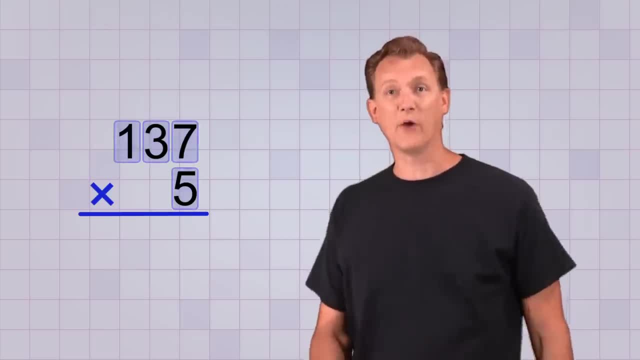 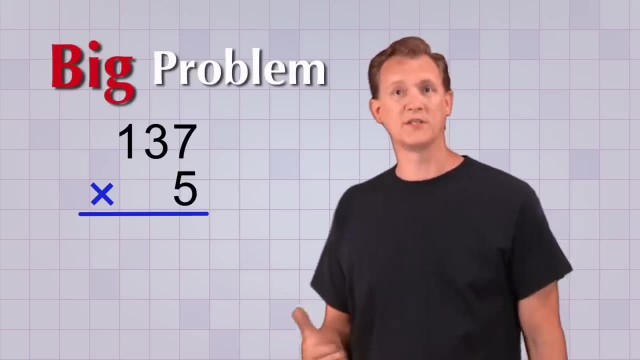 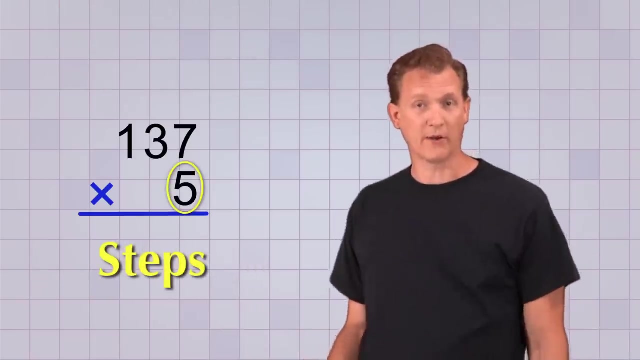 we don't forget that we're multiplying. Okay, now we're ready to learn the procedure for multiplying Basically. what we're going to do is break up this big multiplication problem into a series of small multiplication problems or steps. Those small steps involve multiplying a digit in the bottom number by 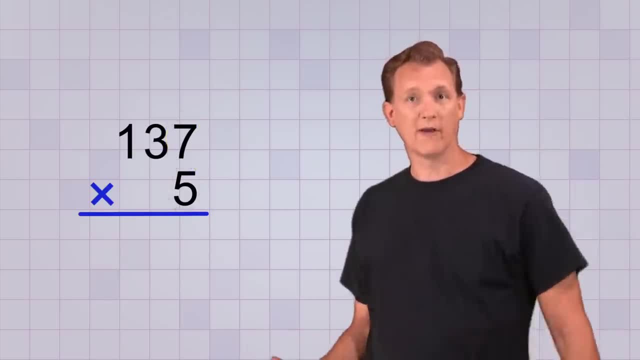 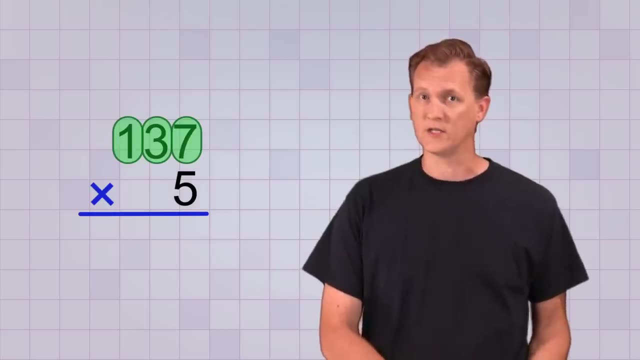 a digit in the top number. Now in our problem we only have 1 digit on the bottom and we're going to multiply it by each of the digits in the top number And since the top number has 3 digits, that means that our problem will have 3 small multiplication steps. 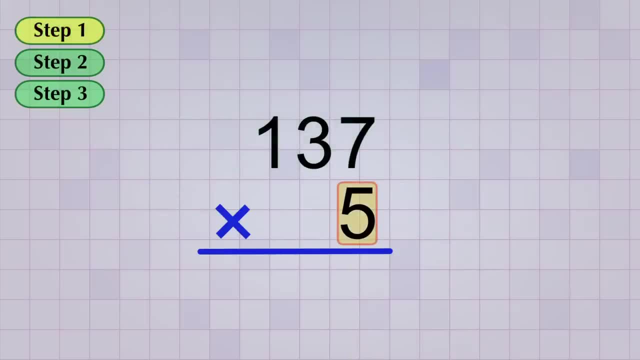 For the first step, we multiply the bottom digit, 5, by the digit in the 1-digit number, Now in the 1's place of the top number, which is 7,. we always start with the 1's place and 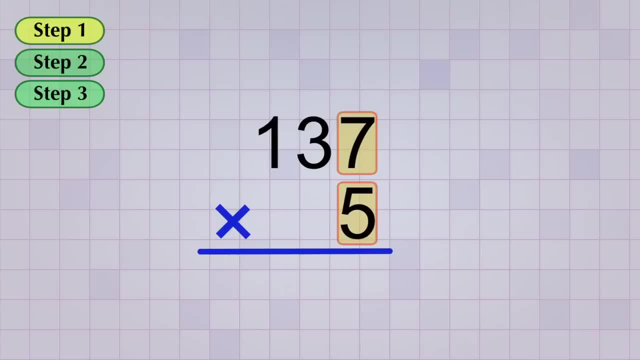 work our way from right to left. So 5 times 7 gives us 35.. Now, just like with addition, when we get a 2-digit answer, we have to carry the first digit to the top of the next column because it'll be in the way of the next answer digit. 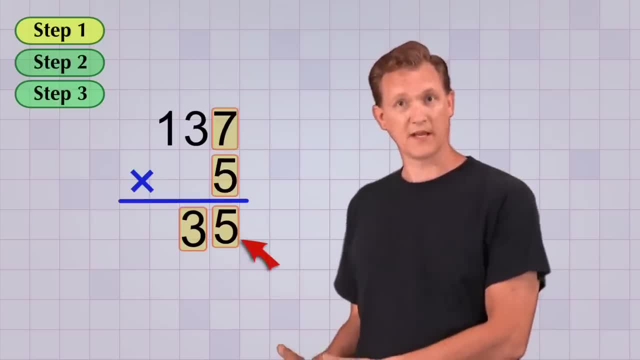 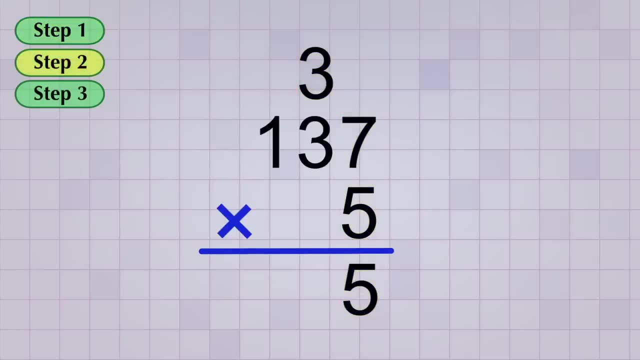 if we don't So, the 5 stays down here in the 1's place of the answer, but the 3 gets carried up to the top of the 10's place column. Now it's time for the second step. We multiply. 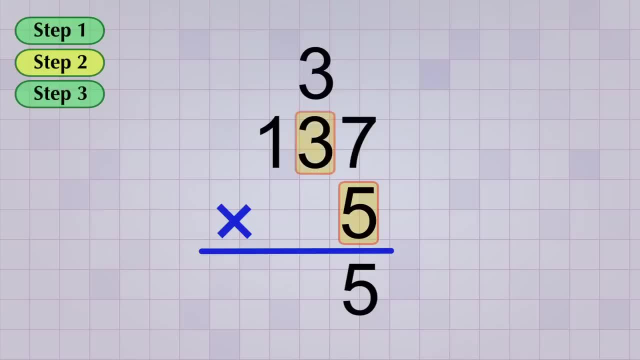 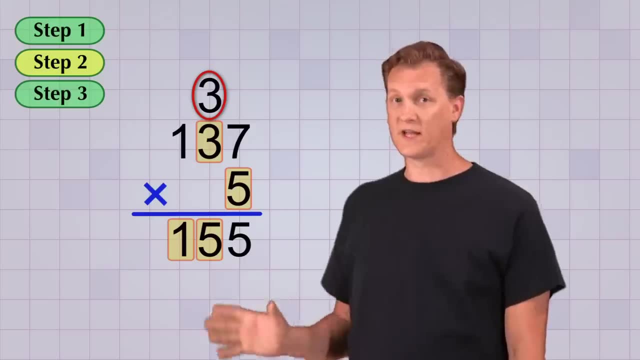 5 by the next digit to the left in our top number, 3.. So 5 times 3 equals 15.. But wait a second. There's that 3 we carried up to the top from the last answer. What do we do with that? Well, we need to add it to the answer that we just got. That's because 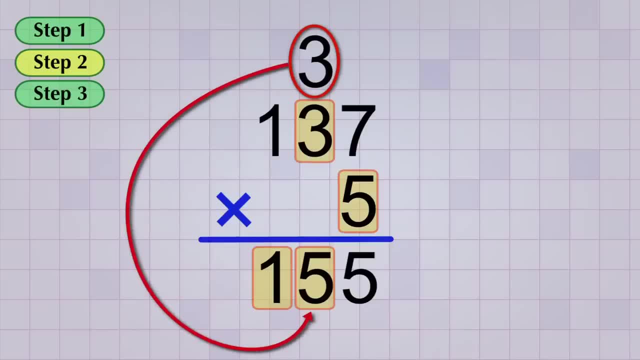 that 3 was supposed to go in the 10's place of the answer, but just not all by itself. We had to do the second multiplication step first and see what else needed to go in that answer spot with it, And it turned out to be a 5.. 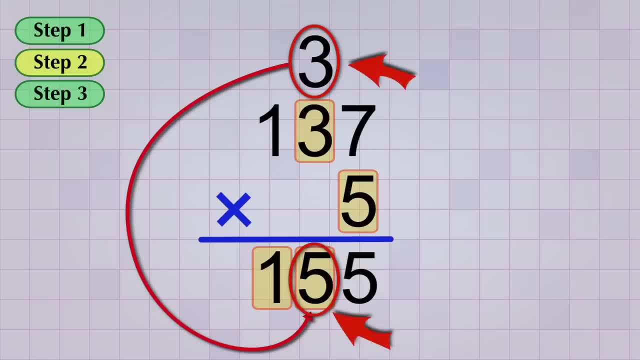 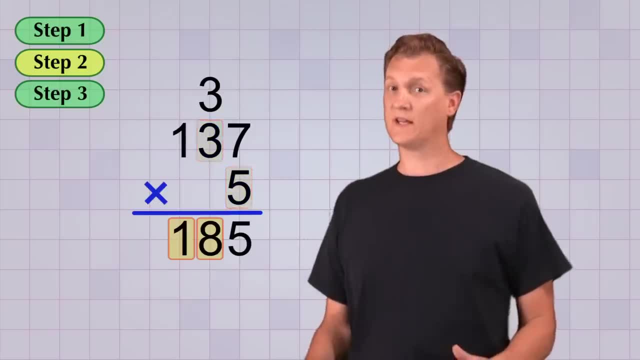 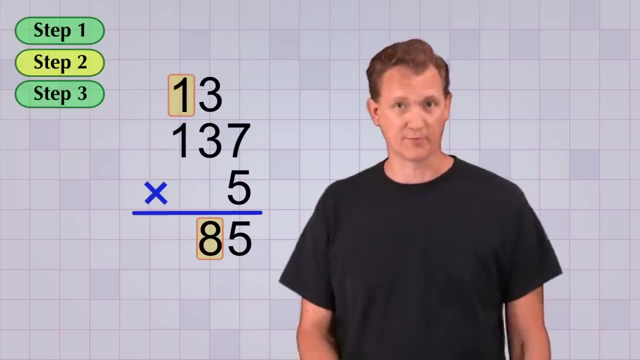 So we have to combine the 2 digits that both go in that answer place. That's why we add the digit we carried and we end up with 18.. But once again our answer is a 2-digit number, so we leave the 8 in our answer line and we carry the 1 up to the top of the 100's. 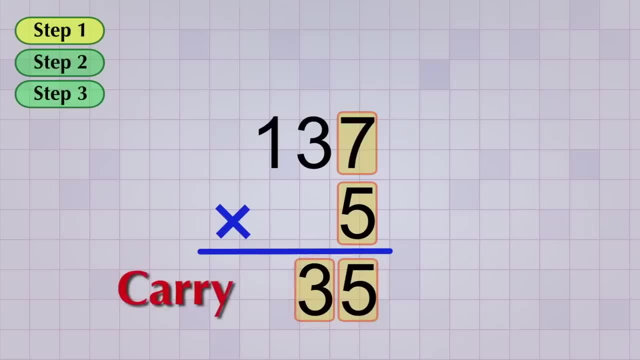 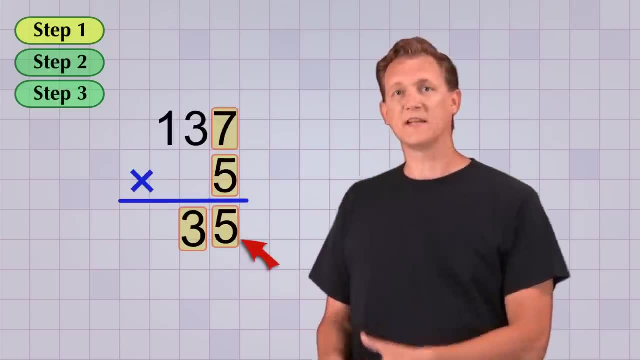 Now, just like with addition, when we get a 2-digit answer, we have to carry the first digit to the top of the next column because it'll be in the way of the next answer digit if we don't So, the 5 stays down here in the ones place of the answer, but the 3 gets. 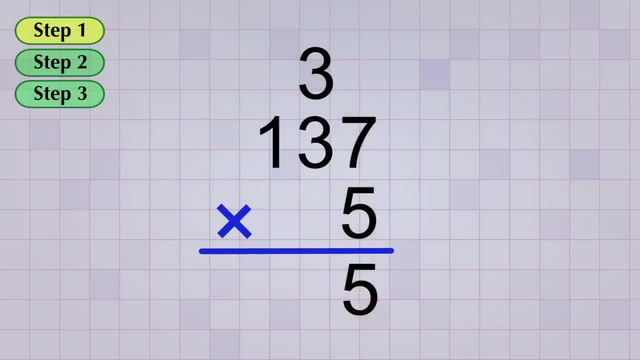 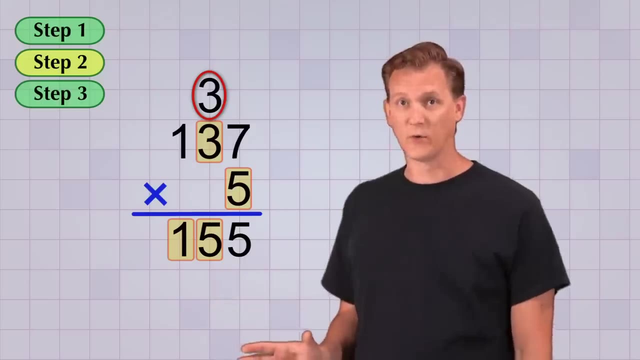 carried up to the top of the tens place column. Now it's time for the second step. We multiply 5 by the next digit to the left in our top number, 3.. So 5 times 3 equals 15.. But wait a second. There's that 3. we carried up to the top from the last answer. What do 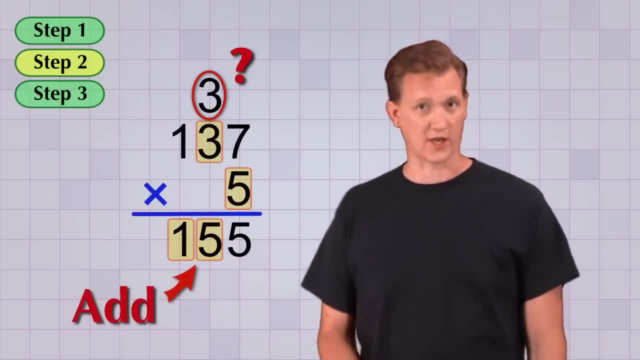 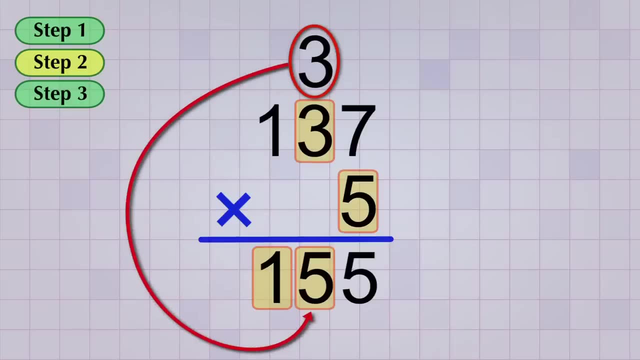 we do with that? Well, we need to add it to the answer that we just got. That's because that 3 was supposed to go in the tens place of the answer, but just not all by itself. We had to do the second multiplication step first and see what else needed to go in that. 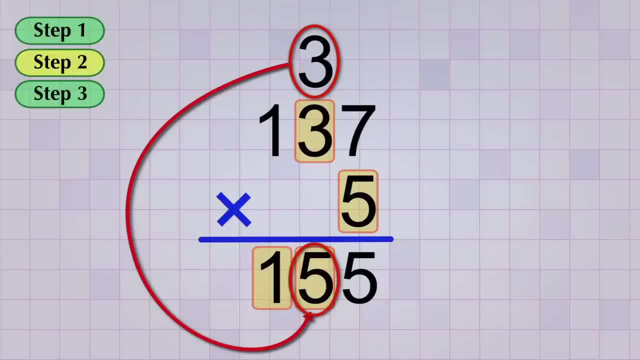 answer spot with it And it turned out to be a 5. So we have to combine the 2 digits that both go in that answer place. That's why we add the digit we carried and we end up with 18.. But once again our answer is a 2-digit number. 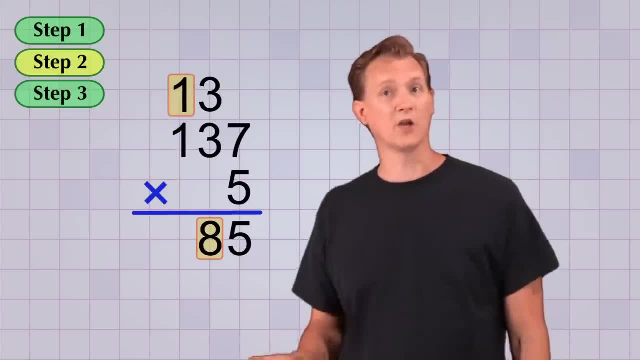 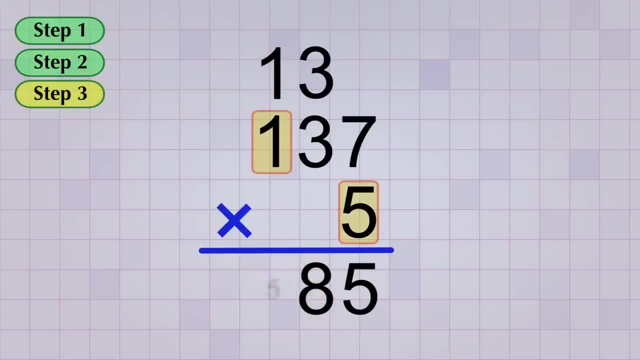 so we leave the 8 in our answer line and we carry the 1 up to the top of the hundreds place column. Now for our third and last multiplication step. We have 5 times 1, which is just 5.. But again there's that digit we carried up above. so it wouldn't be in the way What? 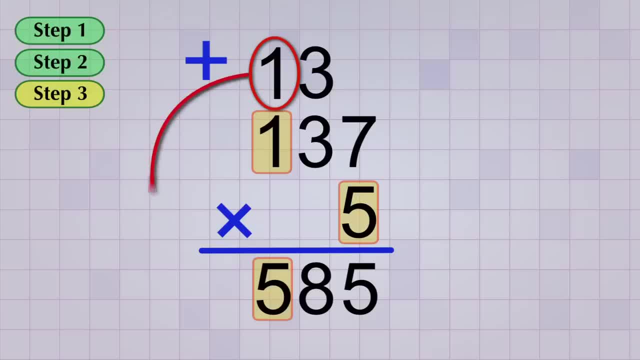 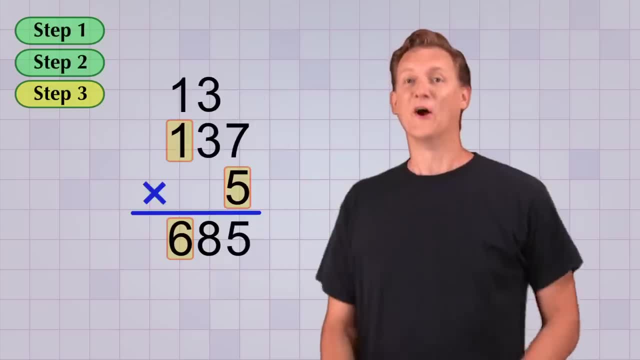 do you think we do with that digit? Yep, we add it to the answer we got from the multiplication step. So 5 plus 1 gives us 6, and that's what goes in our answer line. Okay, then we've done all three of our multiplication steps and the answer to our problem 5 times. 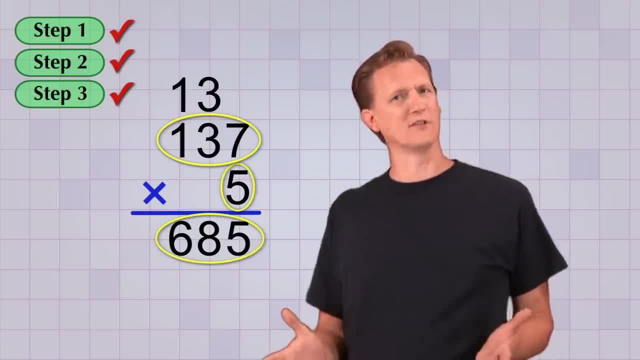 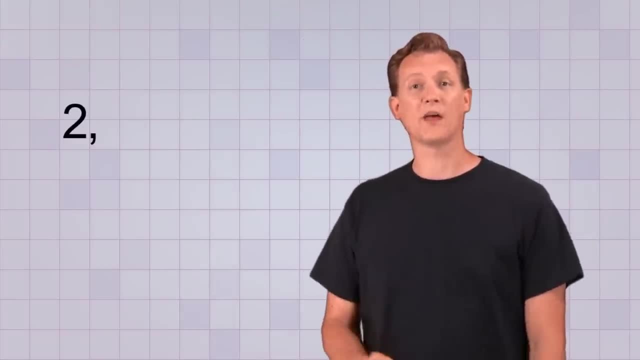 137, is 685.. Now, that wasn't so bad, was it? Let's try one more example before you practice some on your own. Let's multiply 2,617 by 4.. We start our problem with the ones places lined up and we make sure that the number 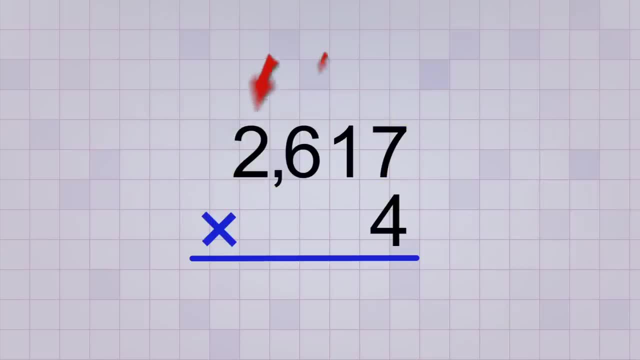 with the most digits is on top, Because our top number has 4 digits. this time it means we'll break this problem up into 4 small multiplication steps. We'll multiply the bottom digit by each digit in the top number, starting with the ones place on the right. 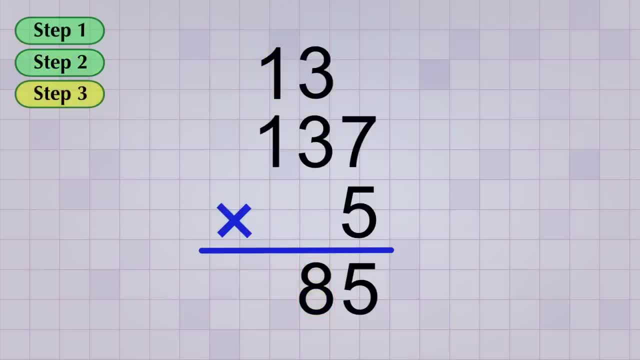 place column. Now for our third and last multiplication step. We have 5 times 1, which is just 5.. But again there's that digit we carried up above so it wouldn't be in the way. What do you think we do with that digit? 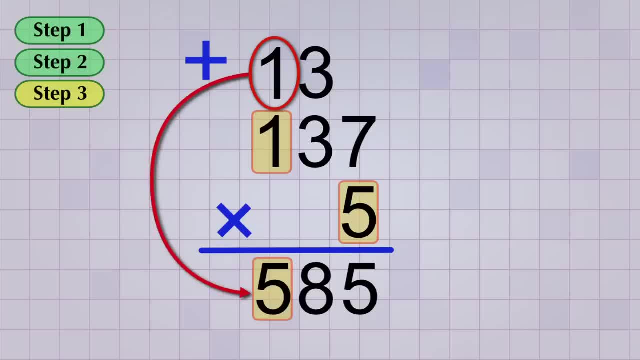 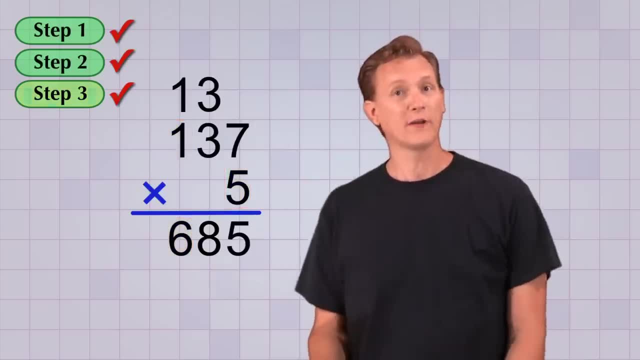 Yep, we add it to the answer we got from the multiplication step. So 5 plus 1 gives us 6, and that's what goes in our answer line. Okay, then we've done all three of our multiplication steps and the answer to our problem 5 times. 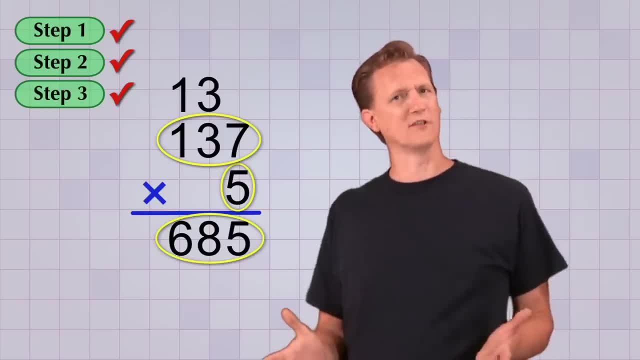 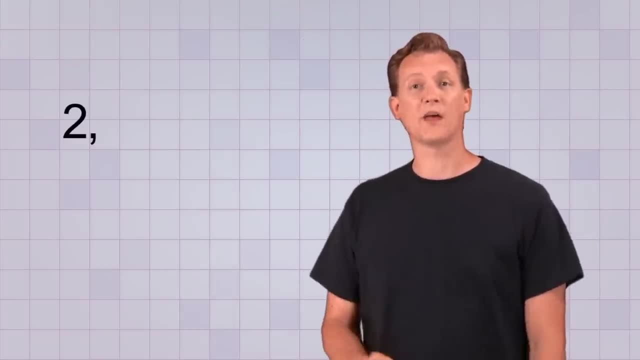 137, is 685.. Now, that wasn't so bad, was it? Let's try one more example before you practice some on your own. Let's multiply 2,617 by 4.. We start our problem with the ones places lined up and we make sure that the number 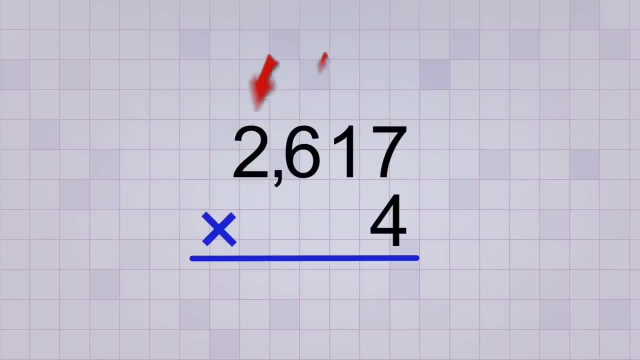 with the most digits is on top, Because our top number has 4 digits. this time it means we'll break this problem up into 4 small multiplication steps. We'll multiply the bottom digit by each digit in the top number, starting with the ones place on the right and working our 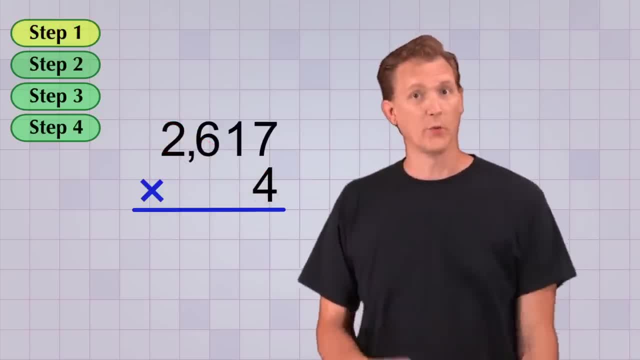 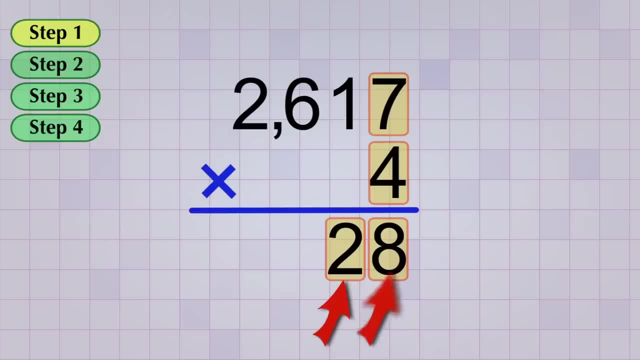 way left. Okay, here we go with the first step. We multiply the bottom digit by the top digit in the ones place. 4 times 7 equals 28.. Because we have a 2-digit answer, we need to carry the digit that will be in the way. We're going to add it back in after we complete. 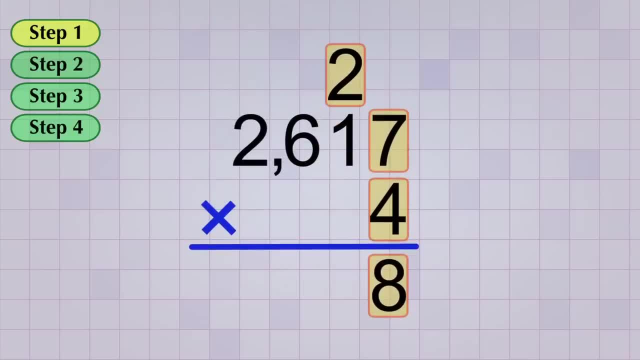 the next multiplication step. So we carry the 2 to the top of the tens column and we leave the 8 where it is. Now we can do the second step. We multiply the bottom digit by the next digit in the top number. 4 times 1 equals 4.. That was easy, But don't forget about that digit we carried. 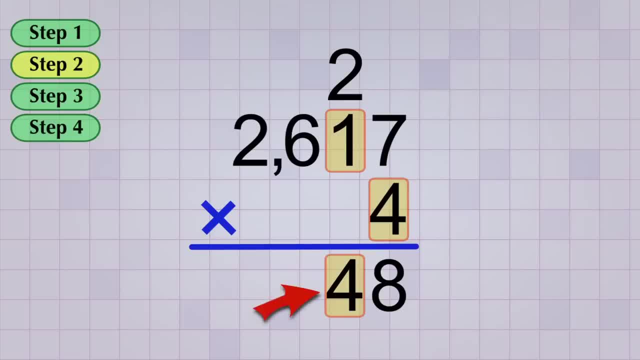 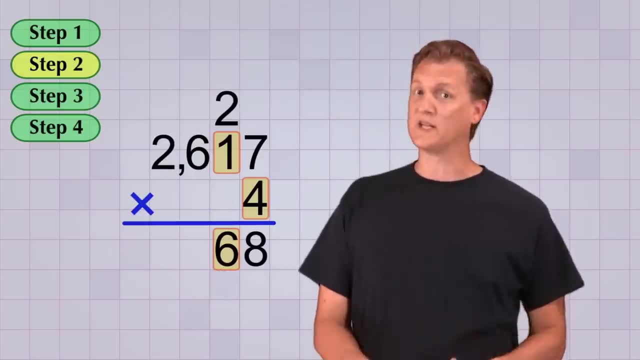 We need to add that to our answer from our second step. So 4 plus 2 gives us 6, and that's what we put in our answer place, And this time we We have a one-digit answer, so we don't need to carry. 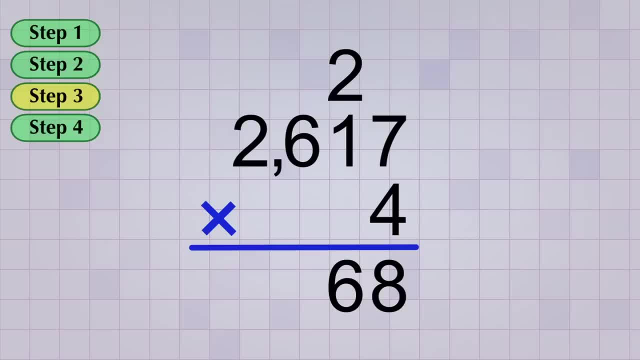 We can just move on to the next step. For our third multiplication step, we'll multiply 4 times 6, and that gives us 24.. Yep, it's a two-digit answer, so we'll need to carry again. The 4 stays in the answer and the 2 moves up to the top of the thousands column.